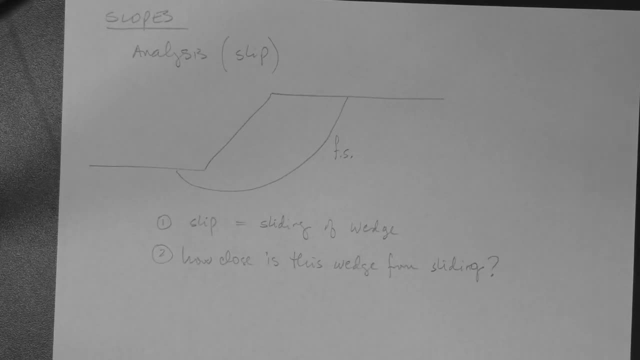 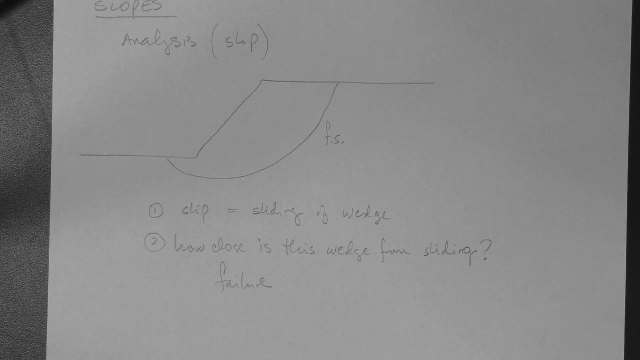 A something that's bad. So we need to define what failure is, but not in the colloquial way or in the general way, but in the theoretical way that is associated with our calculation, Or soon-to-be calculations. Define the failure as the condition where there is an incipient. 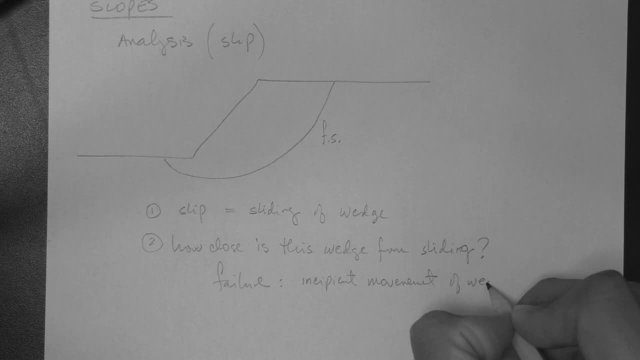 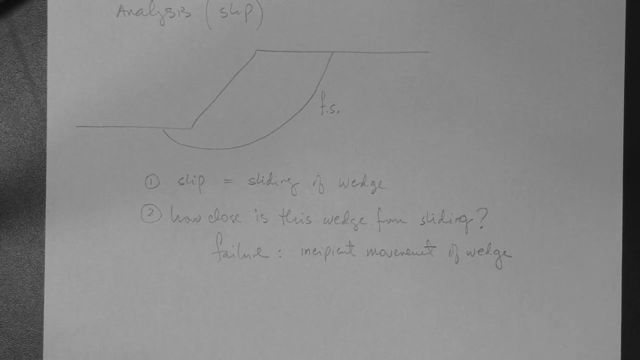 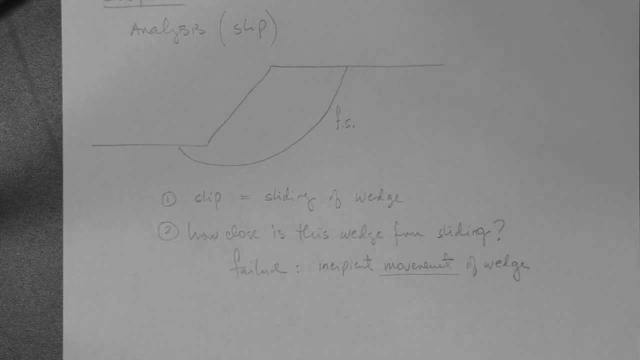 movement of the wedge. So as soon as the wedge begins to move, we consider that situation or that point in time, let's say the theoretical failure. point Now, movement, The movement of the wedge is important. That is the nature of the movement. 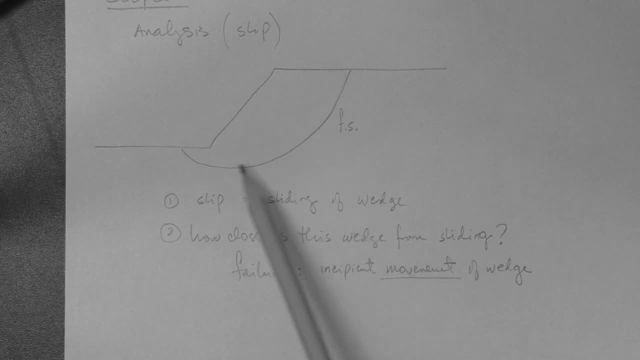 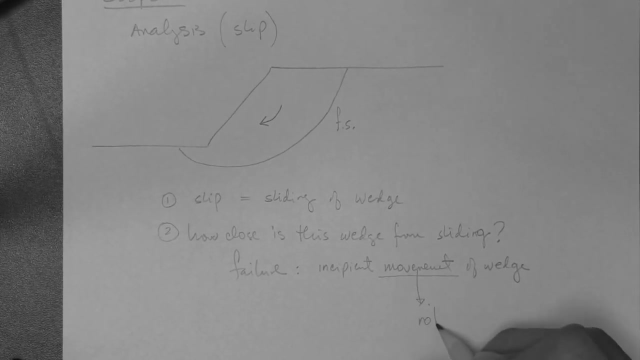 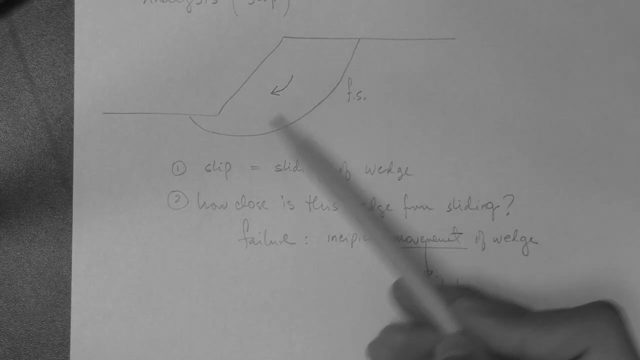 So notice that this particular wedge is resting on a failure surface that is curved. Therefore, the movement of the wedge is naturally going to be a rotation Again. this is because the failure surface is curved. We could have linear, non-curved failure surfaces. 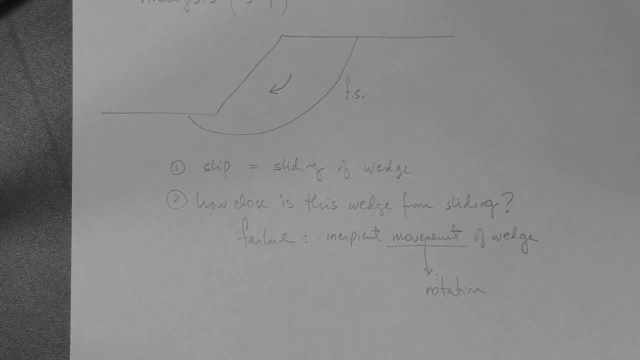 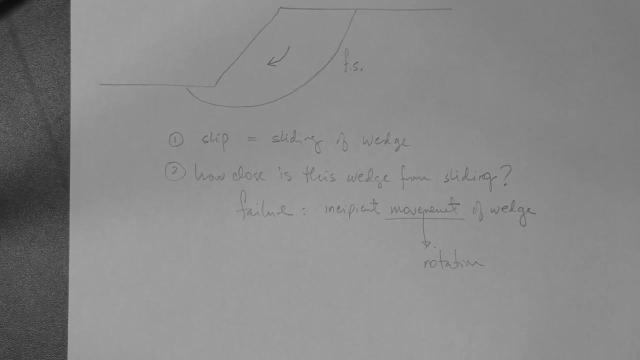 but that will come later. We'll talk about that later on. So if we have a rotation and we are talking about the incipient movement or the beginning of the movement, then we're essentially talking about the point in time where statics in association with moments. 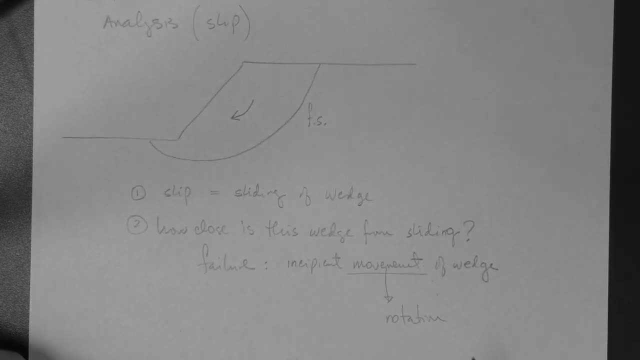 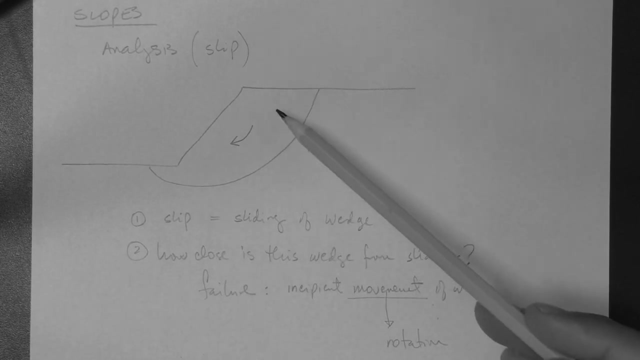 is violated. Now there are two types of moments that are working in this particular problem. There are moments in this system- and we'll calculate them later- that are acting to produce the sliding the slip. These are called the driving moments because they drive the failure. 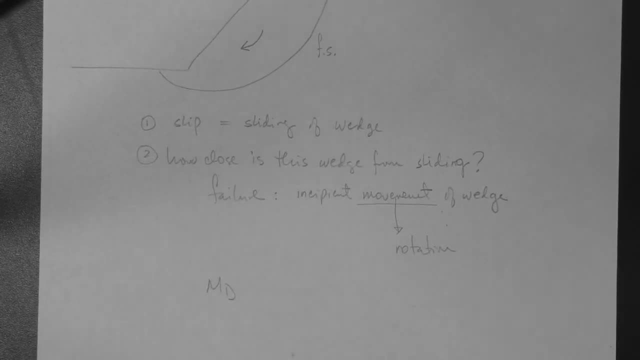 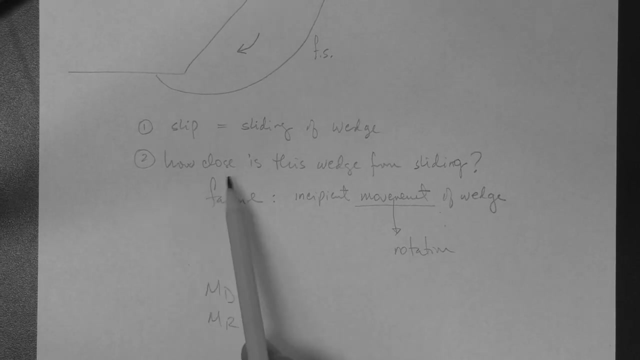 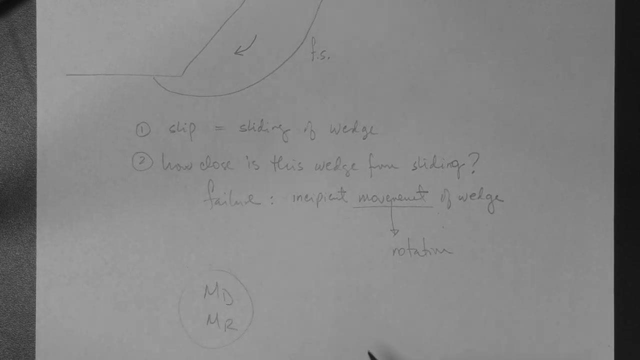 Driving moments And there are also moments that resist the failure And again, we'll calculate these later. So, essentially, the way we answer this question- how close is this wedge from sliding- involves these two moments, And particularly or by definition. 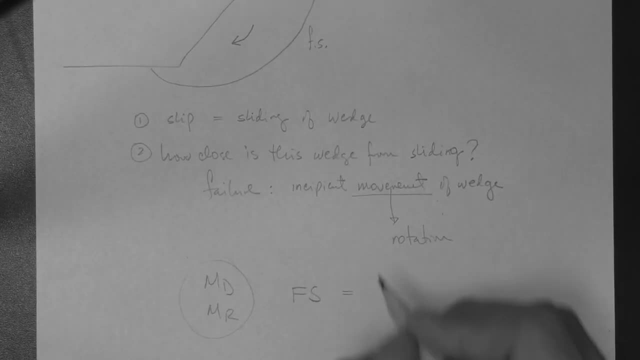 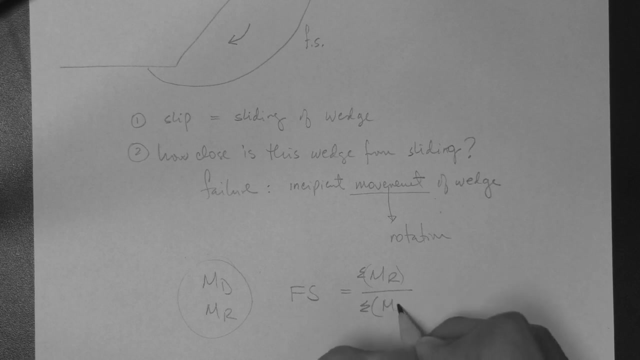 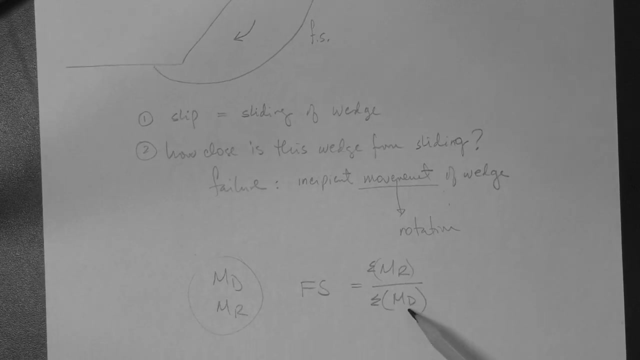 we use a factor of six for safety, which is defined as the sum of the resisting moments over the sum of the driving moments. So this is what happens. We know that if the sum of the moments that are driving the failure, if that sum, 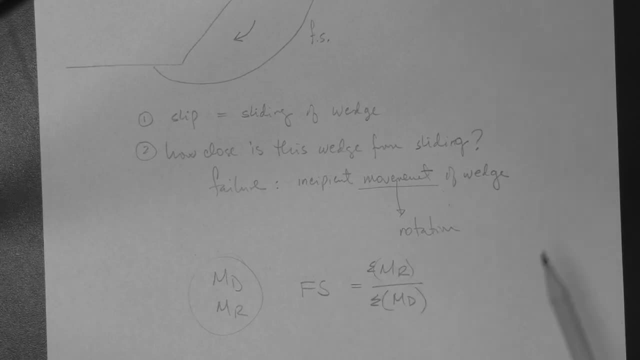 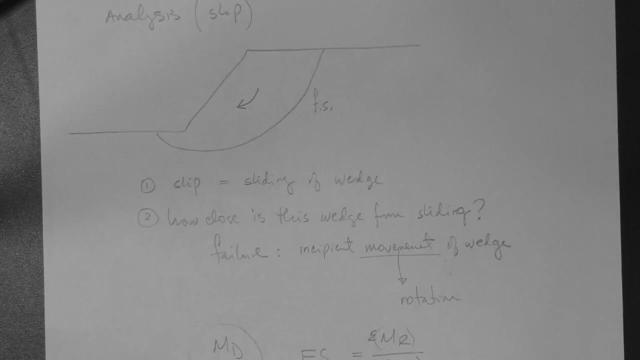 is the same as the sum of the moments that are resisting the failure. if this term is equal to this term, then the factor of safety is one, And we are on the verge of the incipient movement of the wedge That is on the verge of failure. 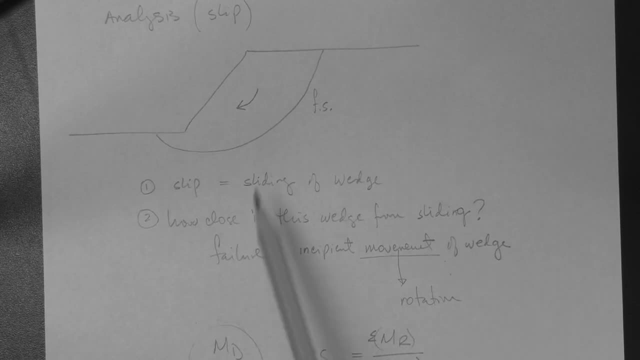 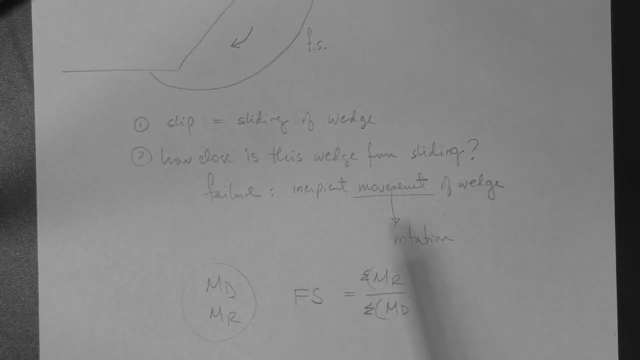 And so factor of safety equal to one means that the slope is essentially on the verge of failure. Now, if, for some reason, we find that the sum of the resisting moments is larger than the sum of the driving moments, then we get a factor of safety. 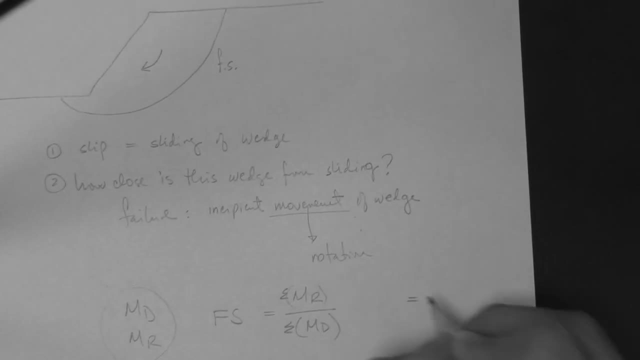 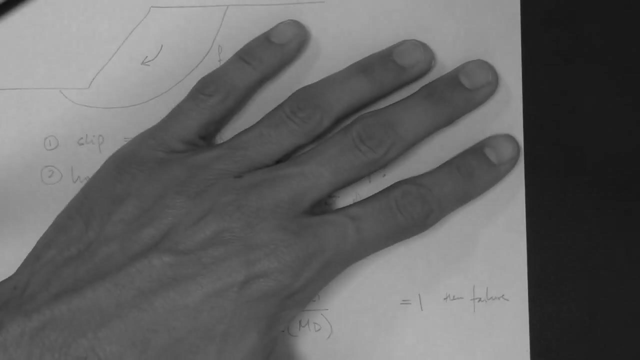 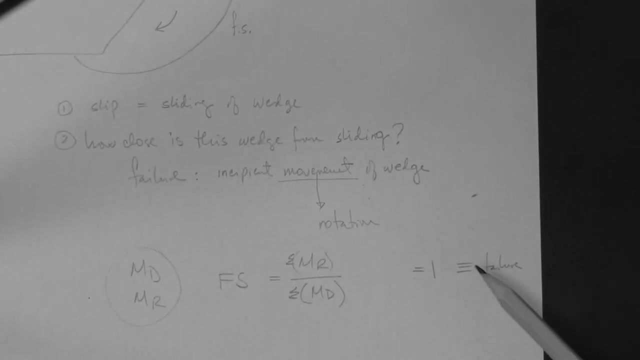 that is larger than one. Okay, So again one, then failure Not then. I mean it really is the definition of failure, or on the verge of failure. I should write here on the verge of failure, but for us. 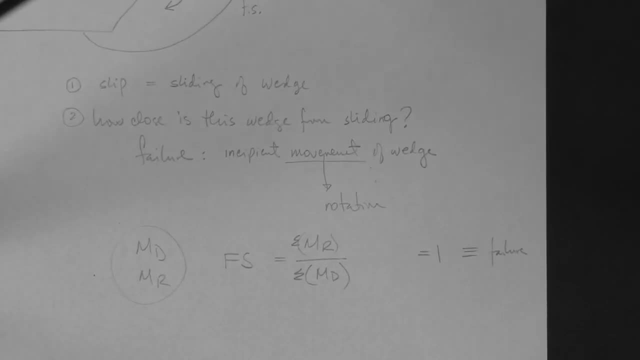 on the verge of failure essentially means unacceptable or essentially at failure. If the factor of safety is larger than one, then we have a situation where the sum of the resisting moments is larger than the sum of the driving moments. Then we have a safe condition. 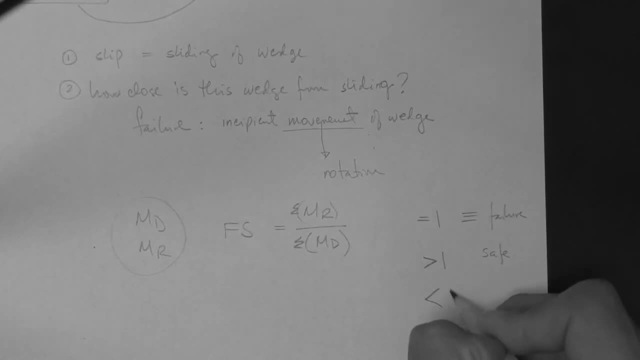 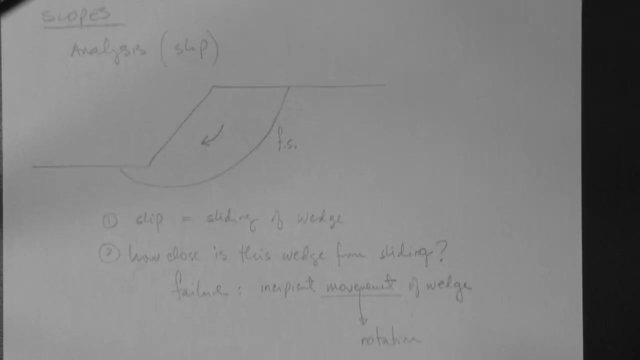 Okay, Now, if the calculated factor of safety is less than one, then we have a situation where the slope that we are analyzing cannot be constructed in the way that is drawn. This is one of the reasons, or one of the situations, that can lead to a factor of safety less than one. 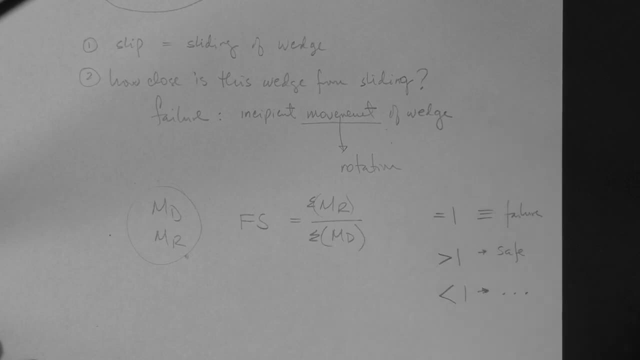 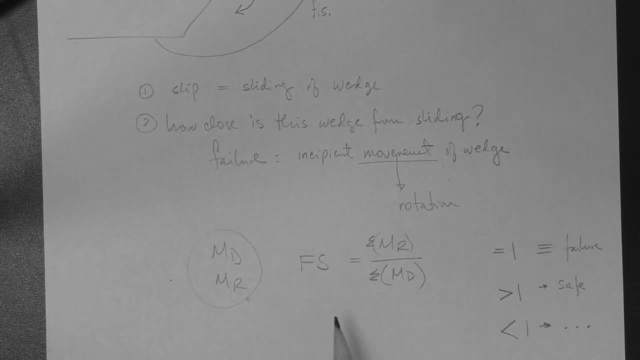 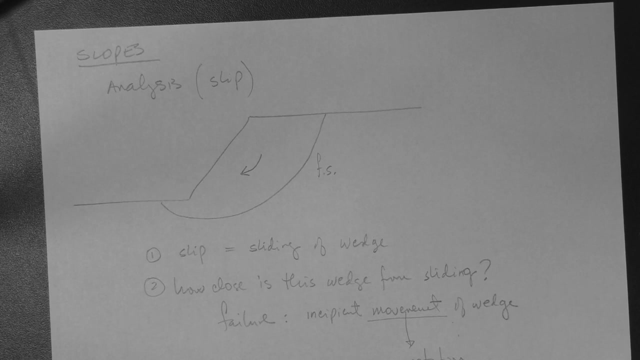 We'll talk about this more later on. It is important to note here that this factor of safety is not the factor of safety for the slope. It's the factor of safety associated with this particular wedge, And we can call that wedge number one. 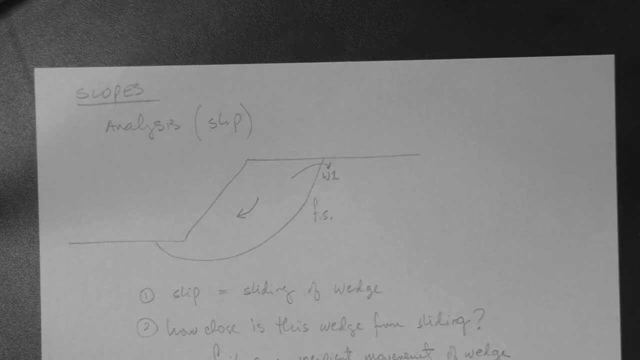 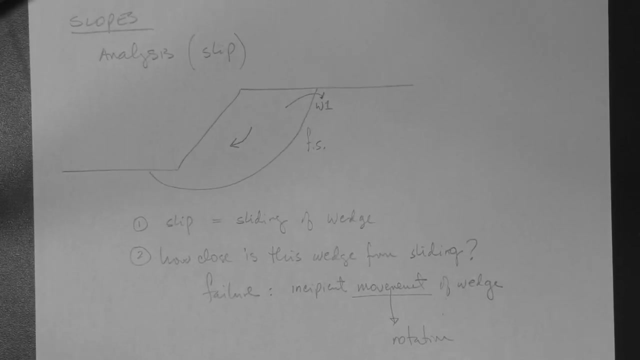 For example, this whole wedge. It's wedge number one. Now you may say, well, is there another wedge? And the answer is yes. There is an infinity of wedges that can be drawn here, So we can proceed down here. 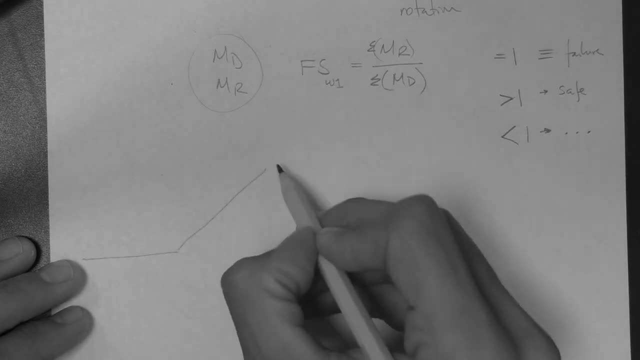 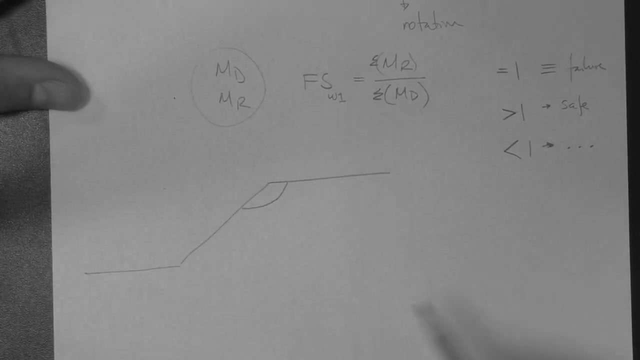 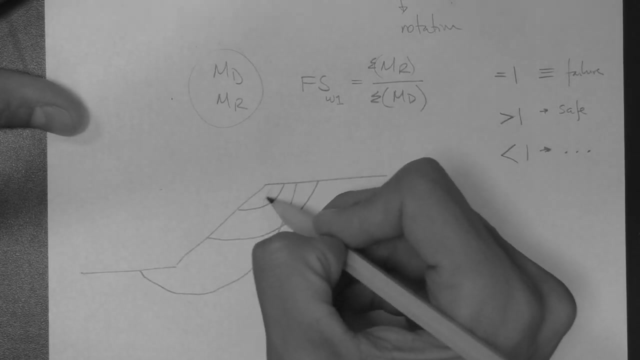 Look, We can draw the slope again and we could find or we could draw various wedges. We can draw small ones like this one, We can draw semi-shallow ones like that or a deep one like this. 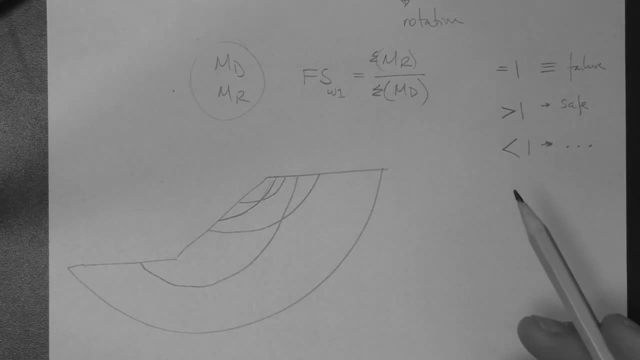 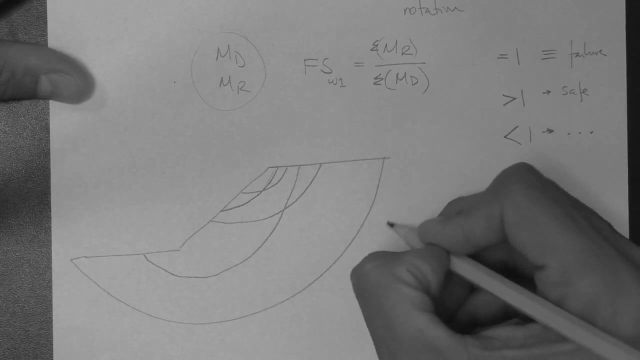 So there is an infinity of wedges that we can draw, And so then the question becomes: in this universe of infinity wedges, which wedge or which failure surface- it's the same question- has the lowest factor of safety? 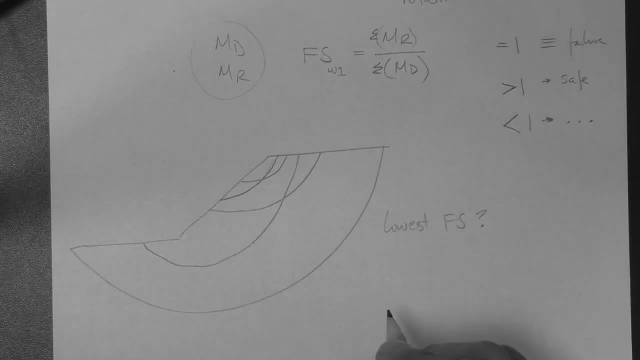 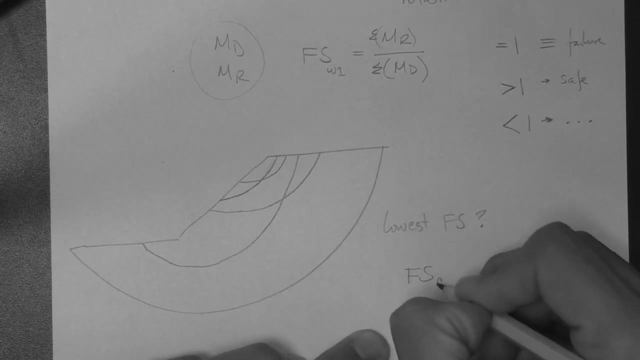 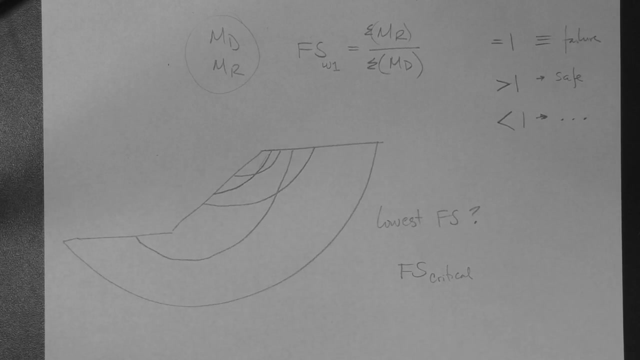 The wedge or failure surface with the lowest factor of safety is considered the wedge or failure surface that has the so-called critical factor of safety, And so we believe that if a failure occurs, it will be defined by the movement or sliding of a wedge. 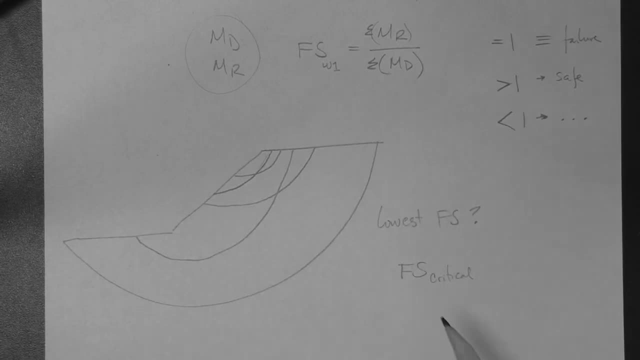 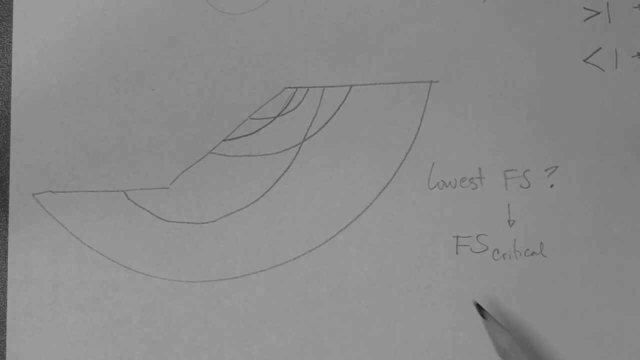 along the failure surface that possesses the critical factor of safety, which is the lowest. And now the question is: how do we determine the critical factor of safety? That is, how do we find, in this universe of infinity wedges, infinity failure surfaces? 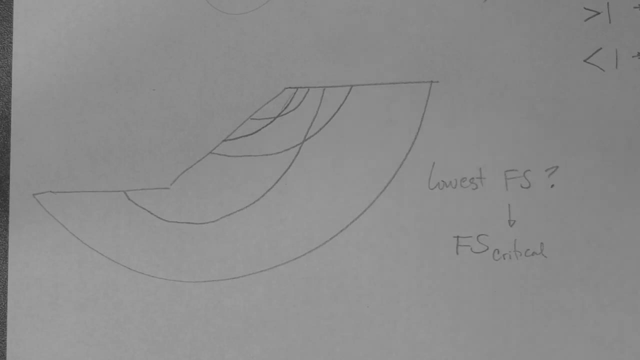 which is the critical one, And so, as you can imagine, we attempt to do this with a computer, because a computer is able to analyze a large number of failure surfaces or wedges very quickly relative to our ability to do it by hand.